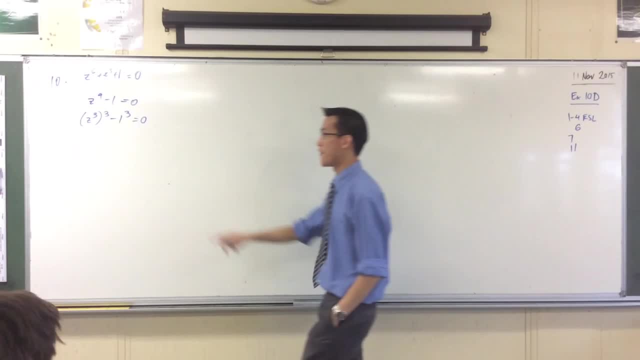 This isn't just you remember. I showed you a bit of a fancy trick for factorizing z to the 9 minus 1.. Do you remember that? Or z to the n minus 1.. We said this: z to the n minus 1 is going to be z. take away 1,. 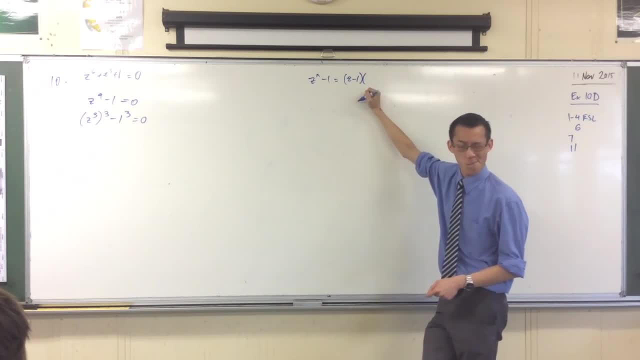 times. do you remember what comes in next? It's the gp. It's the gp. It went 1 plus z plus z, squared, plus dot, dot, dot dot all the way up to z to the n minus 1.. Okay Now, this is not a bad thought to have. 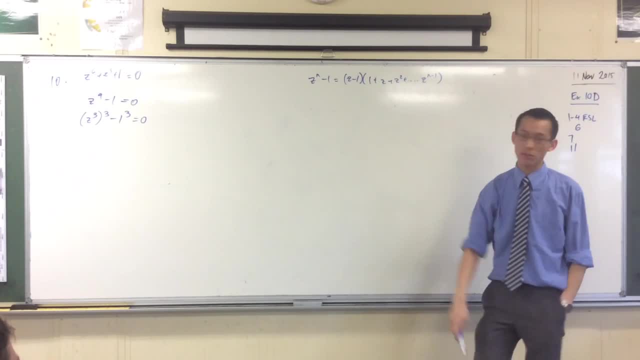 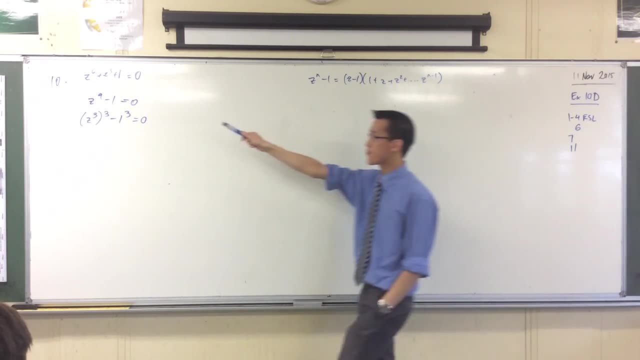 Like I need to factorize in some way. but you can see it's not going to give us the answer that we need, because look how many z terms I have over here. If I were to do this guy, I'd have um. 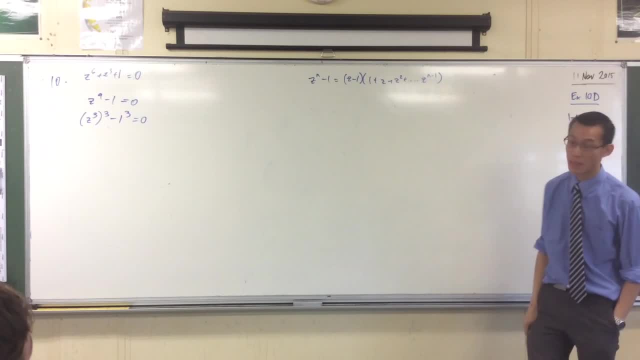 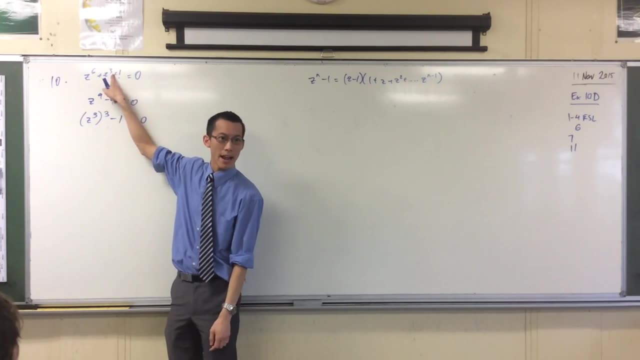 1 plus z plus z, squared all the way up to z to the 8.. Okay, And also, not only am I going to go all the way up to z to the 8, but I'm going to have every one of the terms right. 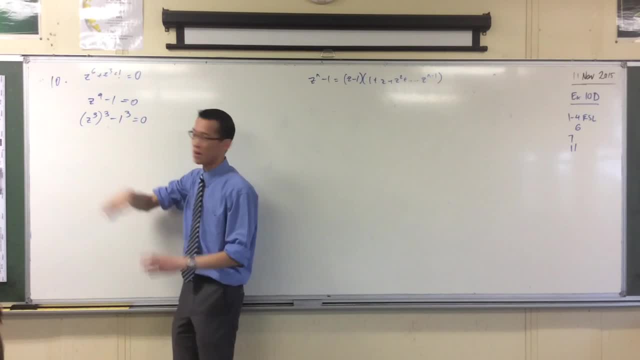 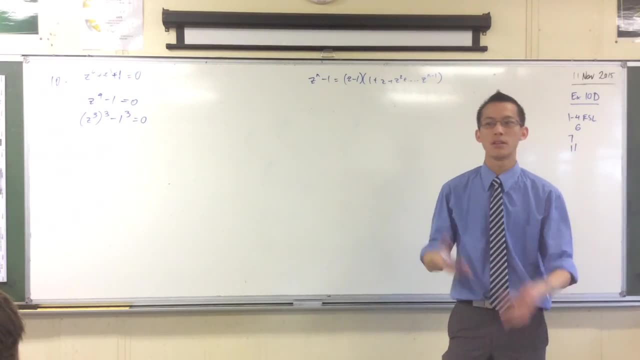 Every power of z will appear, Whereas here I'm missing a whole bunch, right. So that's kind of no good, and that's why I leap towards: okay. what other factorizations can I use? Difference of cubes, Okay. 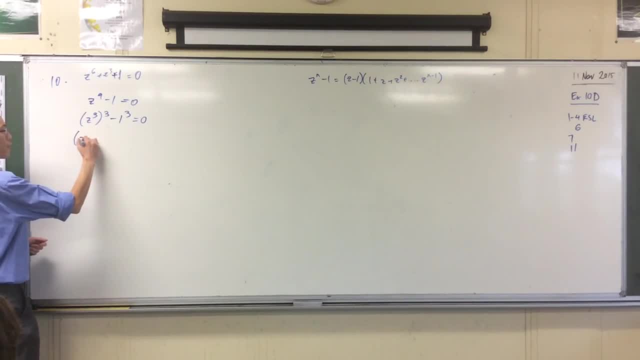 So let's write the factorization for difference of cubes here. Out the front I've got z cubed minus 1.. Okay, There's that term there. And then what do I have over here on the right-hand side? Okay, so it's usually. 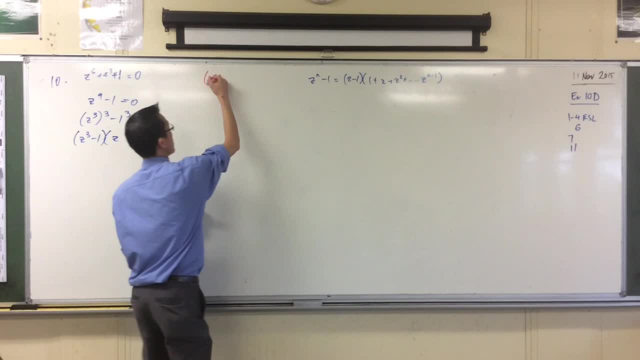 like. let me just write this on the side. Usually my difference of cubes looks like this: Um, if I did say: um, oops, a cubed, take away b cubed. our usual factorization is same opposite. 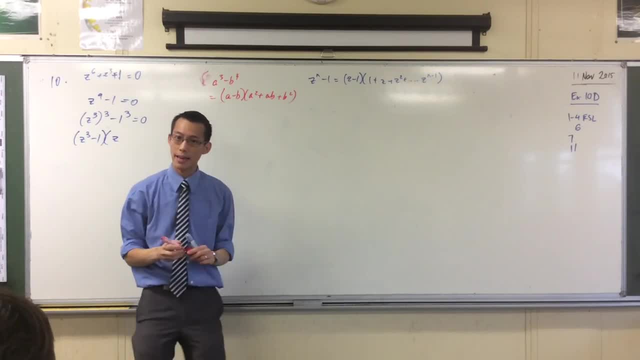 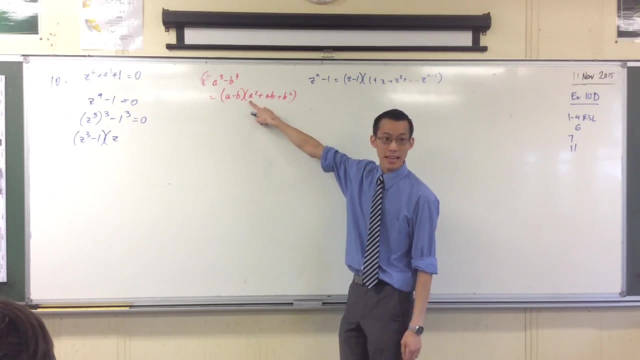 uh, a, b always positive, right, You see that? Okay. Now, being that the thing that's being cubed at the front is itself z cubed, then the next thing that comes along is z cubed squared, z cubed squared. 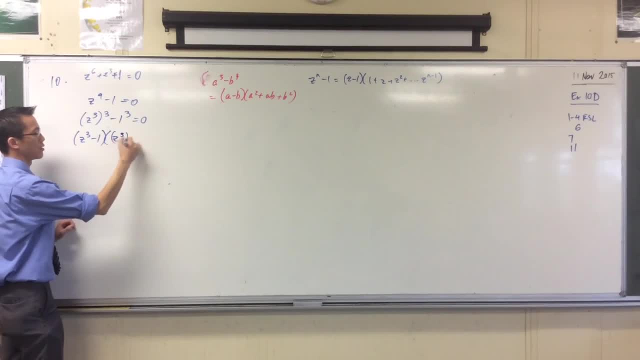 You see that. So that's why, in fact, I'm even going to write that z cubed squared, so that you can see where my z times 6 comes from. Okay, My next bit is a, b, which is just 1 times z cubed. 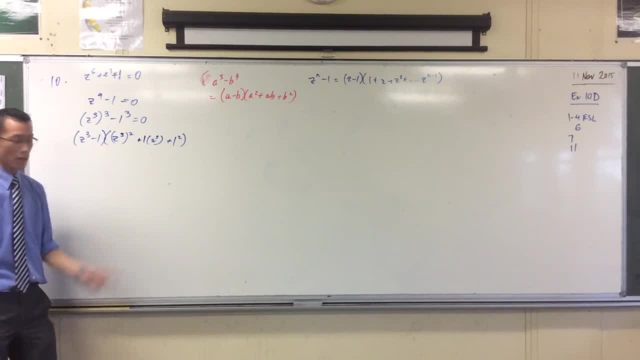 and then my last guy is 1 squared You okay with that? So there is the piece that I was after, right? So this whole thing is equal to 0, because I've just factorized that, I've got. 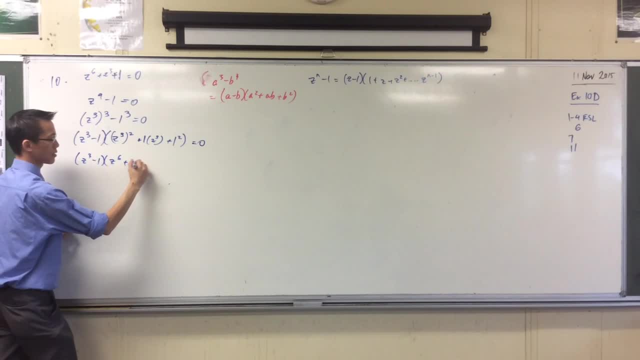 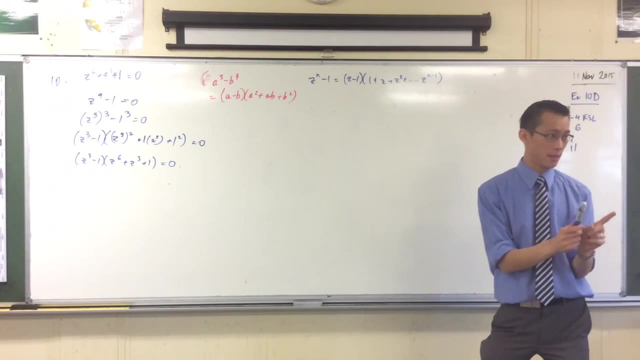 z cubed minus 1, and here is my z to the 6, z cubed plus 1,. happy times. Now, what's the point of that? Okay? Well, when you factorize something, the whole point of factorizing. 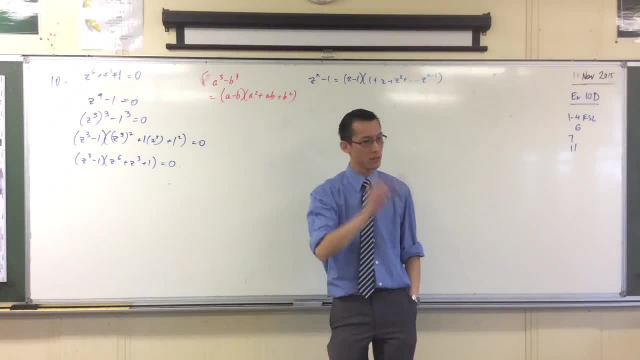 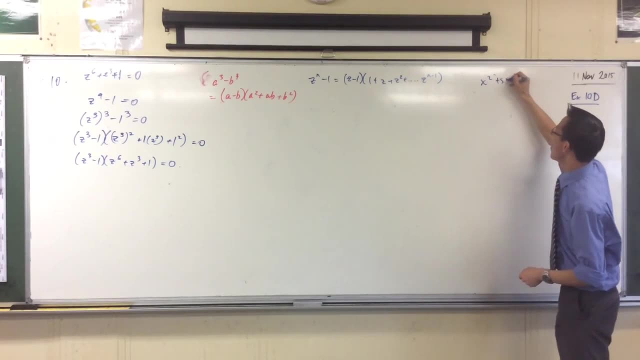 is that if you have 0 on the right-hand side, then the solutions to each of the factors are solutions of the original thing, Right? So, for example, when you have a quadratic and you factorize, okay, the whole point is that once you've got these factors, 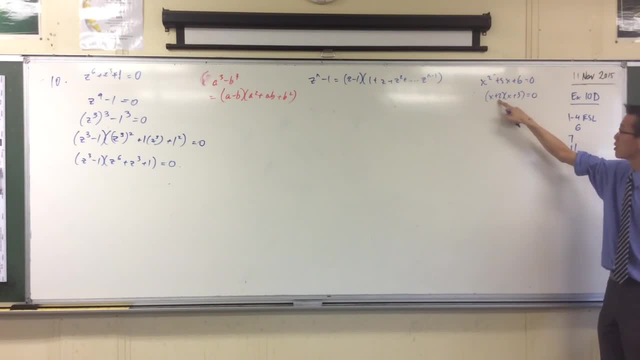 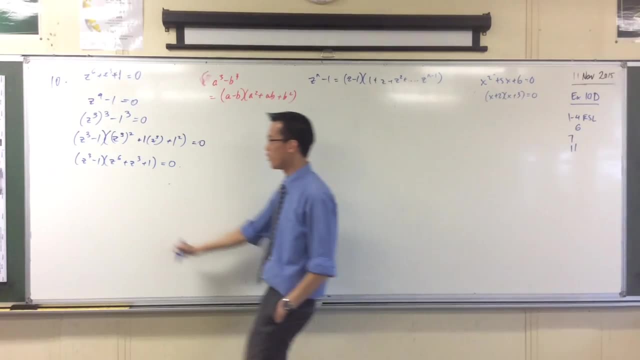 right. if there's a solution for this, that solution will also solve this guy right, And if you've got a solution for this, it will also be a solution of this guy, okay. So therefore, the solutions of z to the 9 minus 1. 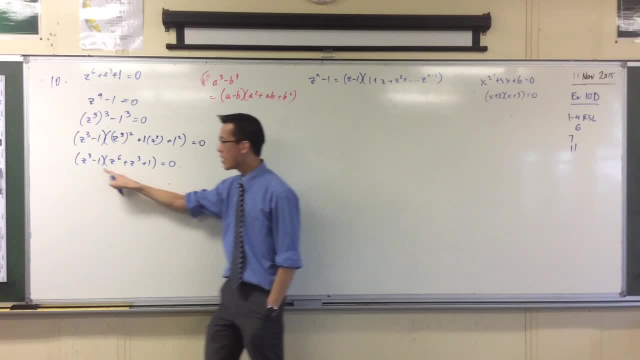 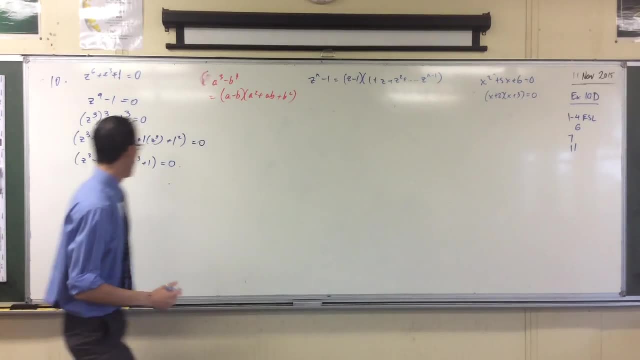 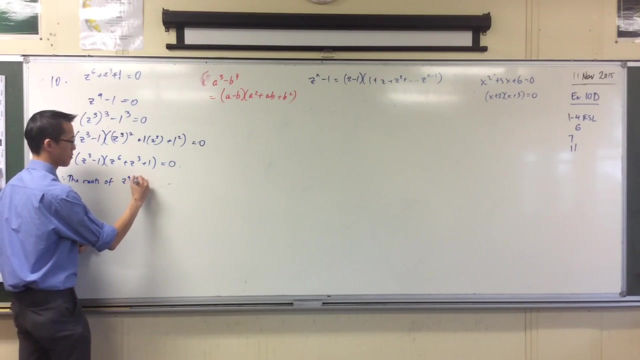 are here and here. okay, So everything that solves this will solve your original, and everything that solves this will also solve your original. okay, So I can say, therefore, the roots of z to the 9 minus 1, z to the 9 minus 1. 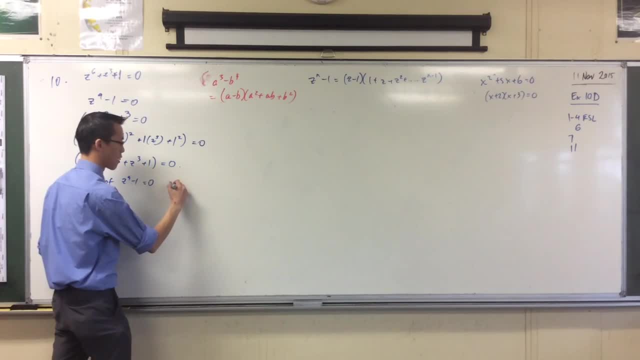 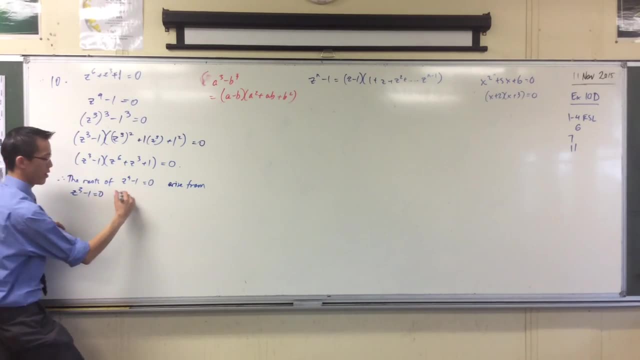 equals 0, come from or arise from these two factors: right, z cubed minus 1 equals 0, and z to the 6 plus z cubed plus 1 equals 0.. That's all you need to say. You're finished, okay. 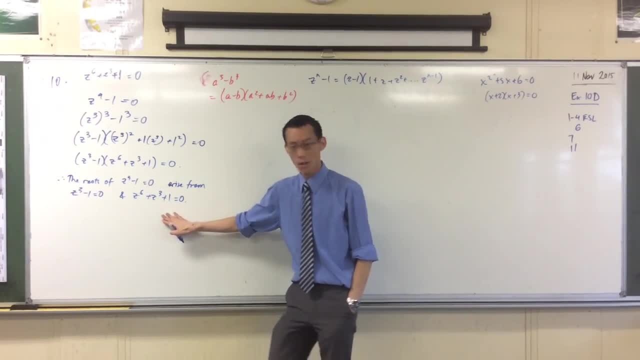 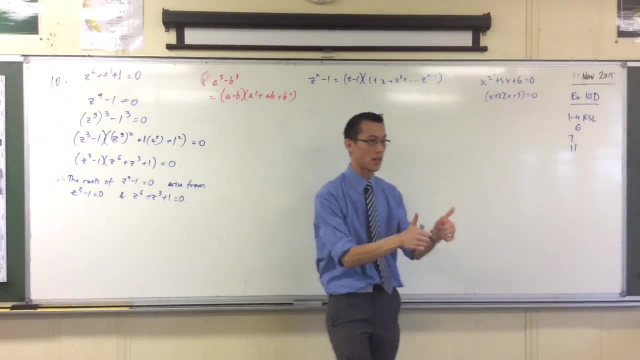 I've established that this and its solutions will be solutions to this, which is all they were asking for. right, Show that the roots of this guy are roots of this guy. Happy times. okay, Have a look at the next part. It's an easy part visually. 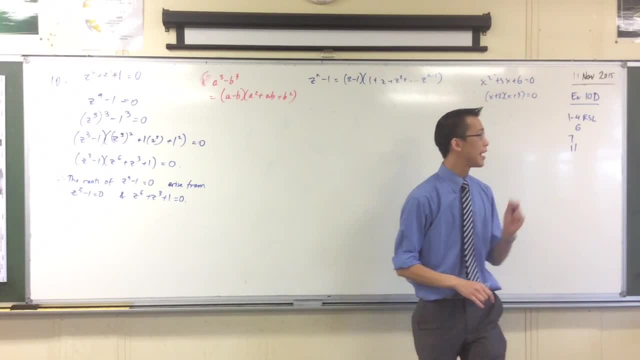 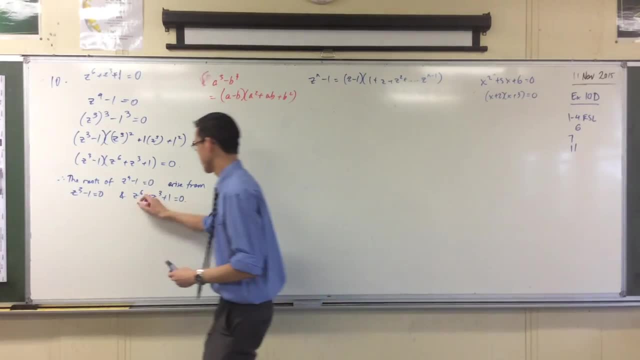 Show those nine roots on an Argand diagram, Identify which one of them's, which ones of them are the solutions to this. Okay, so let's just draw a quick Argand diagram. What is 9 and 9?? Okay now. 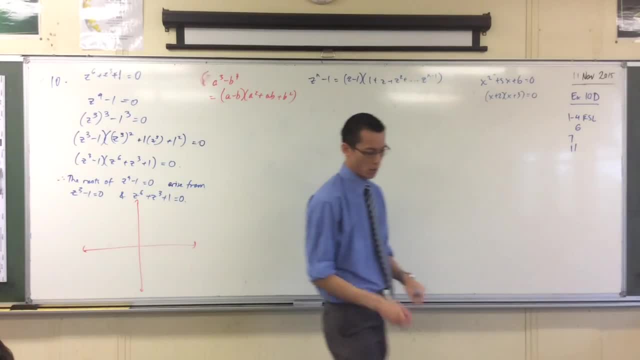 because we're talking about roots of unity, and unity is a real number. what do I know about these nine roots? So 2 pi divided by 9?? Yes, that's right, They're 2 pi on 9, spaced out around the circumference. 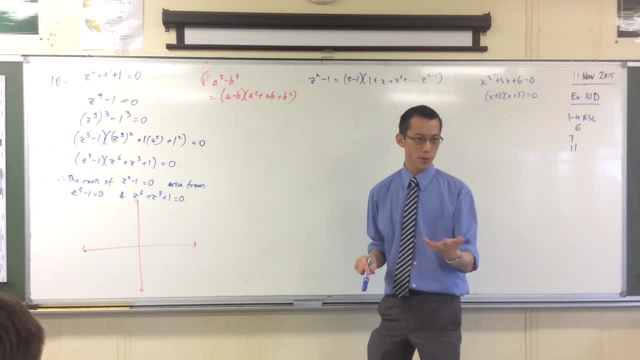 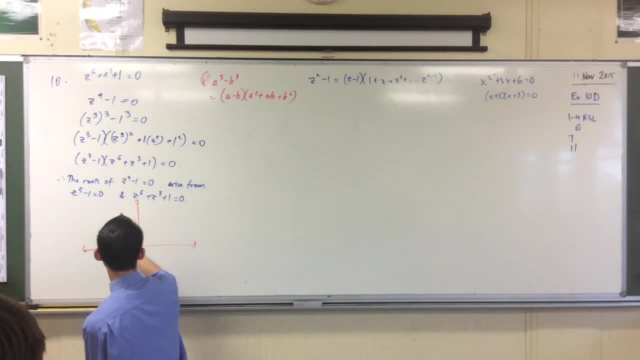 And also because of the complex conjugate root theorem- and one's a real number- they're all going to be paired up as conjugates, okay. So I'm going to start with: let's draw a unit circle. Okay, My first solution of unity. 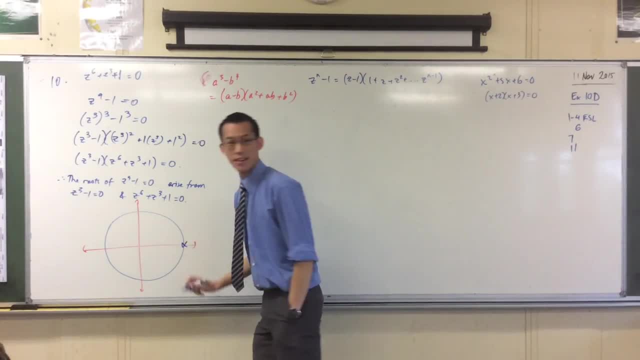 is always unity itself. Slap that guy there Now as I draw the rest of them out. okay, I need to fit. there's my first solution, and how many solutions am I going to have? in total, Nine For the nine roots of unity. 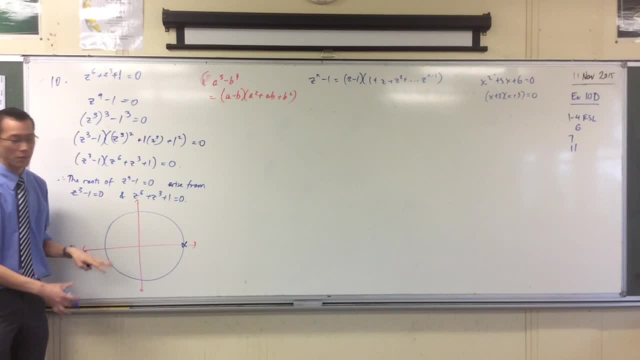 I will have nine in total, So I've got another eight to draw on here. okay, So I know roughly where they're going to fit. 2 pi on 9, which is the next one up? 2 pi on 9,. 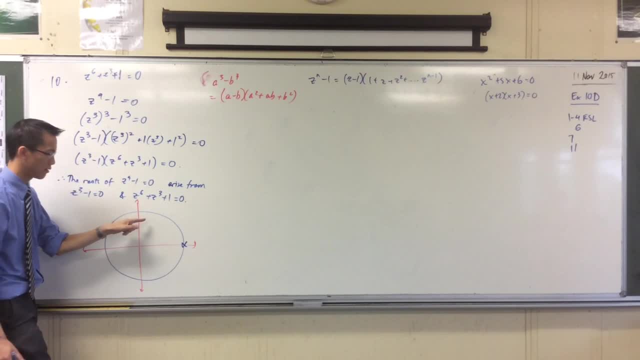 where's that? That's going to be roughly. am I going to fit two before here? Three, six, seven, eight, nine, That'd be so over here. I'm going to go one here and one here. They're going to just fit. 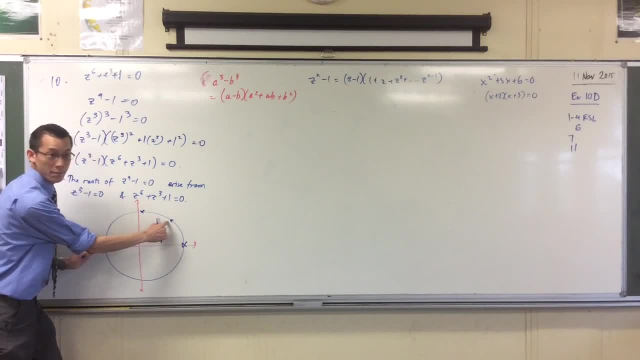 before pi on 2, because this will be 2 pi on 9,, right, This will be 4 pi on 9.. What is what's right on there in terms of on 9?? It'll be 4 and a half pi on 9.. 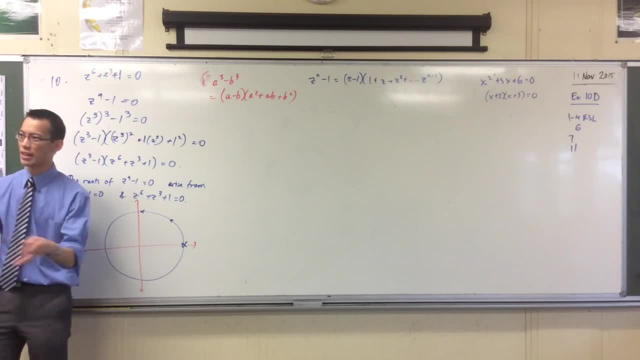 Do you see that? That's pi on 2.. Okay, so that's why I judge, Like I'm just trying to give you practical tools for like, where roughly do I place these? And then I'm just going to keep going around. 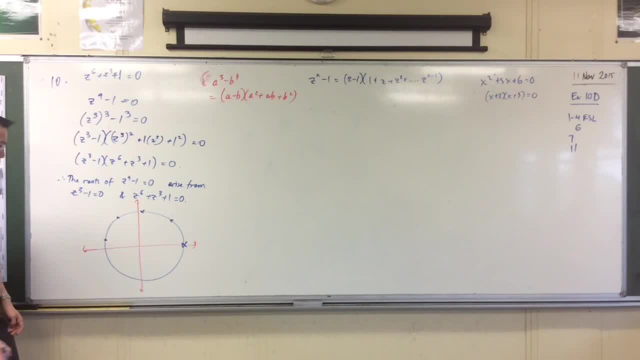 So there's my third one and there's my fourth one. Okay, Or fifth, depending on where you count. Okay, One, two, three, four, five. I've done all of the ones for a positive principle argument and clearly I can't go any further. 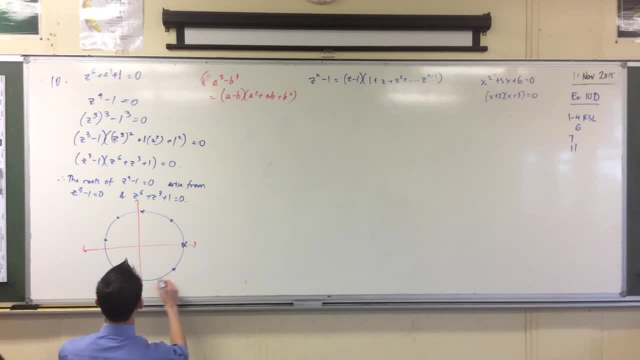 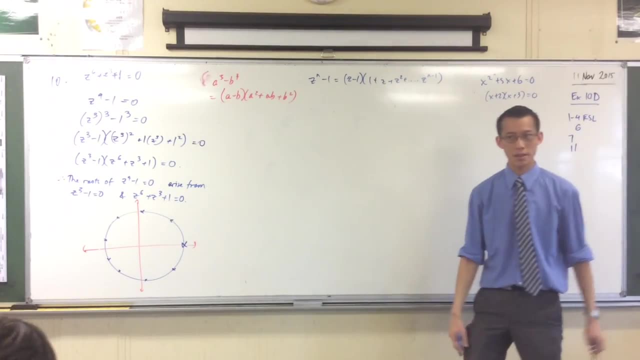 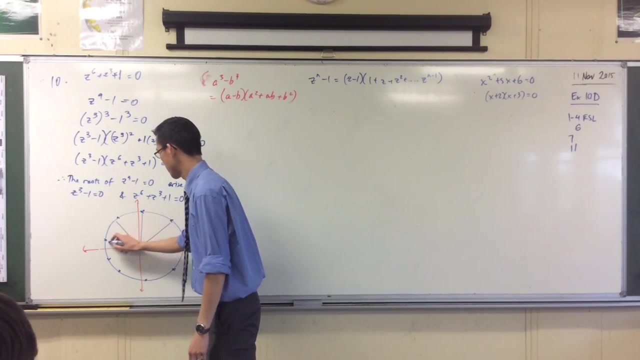 So now I just do all the conjugate pairs like so, Okay, roughly right Now there are all the ninth roots. okay, And I'm just going to quickly. I'll draw the lines up to each one. Is it bad if you're like: 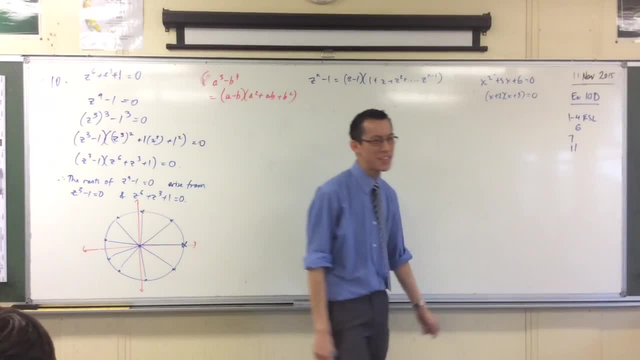 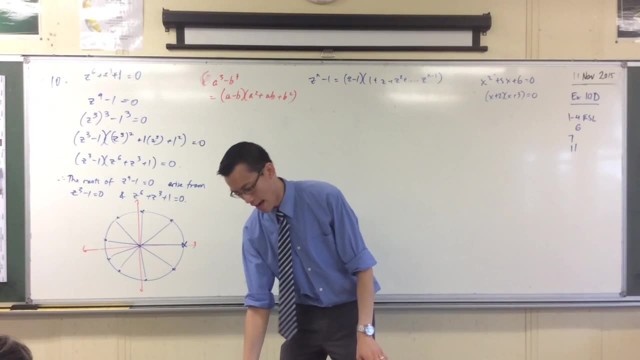 not that accurate. If this were an actual question like this- was this appeared in an exam- you would need to like. what I would do is I would get my calculator out and I would say: okay, what is what is 2 pi on 9?? 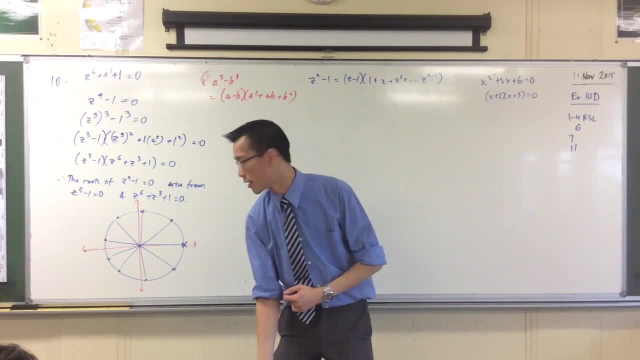 And then it's going to be a certain angle, and it doesn't have to be precise, but it has to be enough that, for instance. I mean, the classic problem is we do these roughly, okay, and then by the time you get to here, 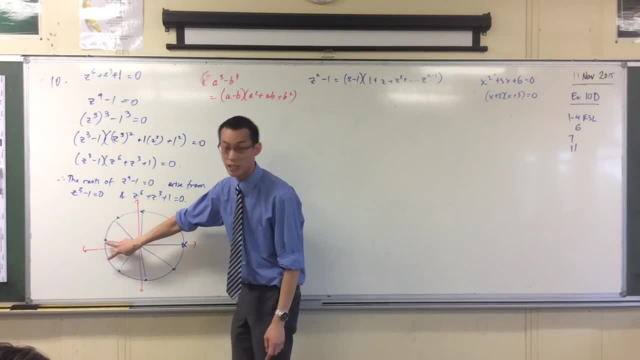 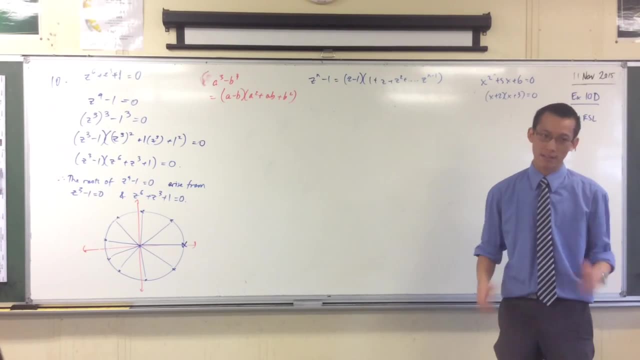 you've your. your estimate's been so far off that these two clearly do not look evenly spaced along with the rest of them. So I actually don't think it's that bad an idea to actually properly bring in a protractor so that you can like. 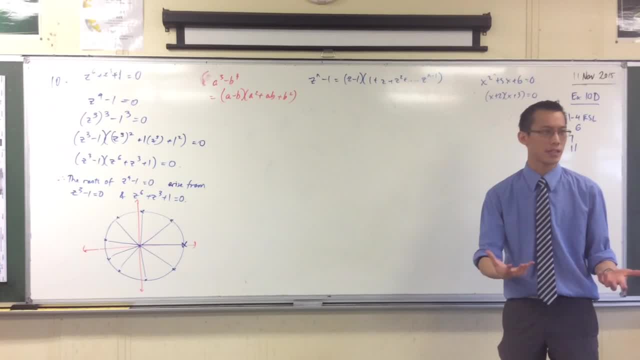 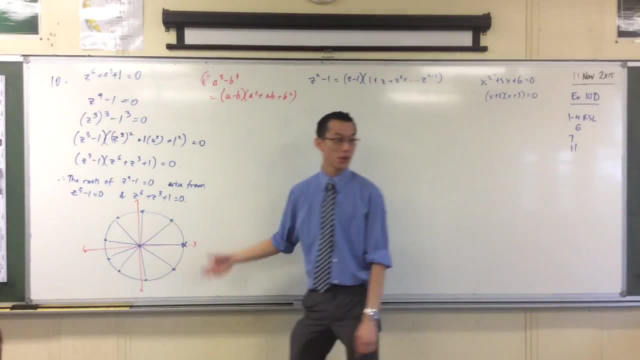 roughly, at least within like plus or minus, say, five degrees. pop it in the right spot and have your. that would make a nonagon. I think it's called a nonagon. Yeah, That would make your nine-sided regular polygon. 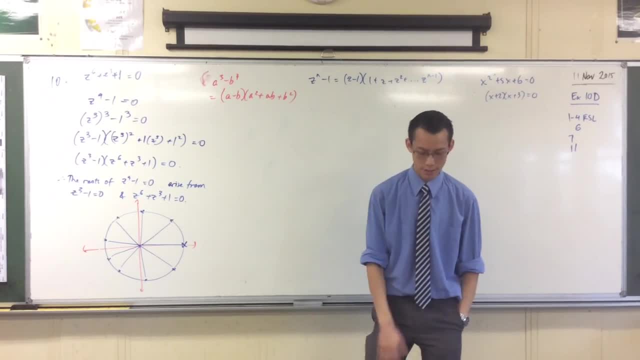 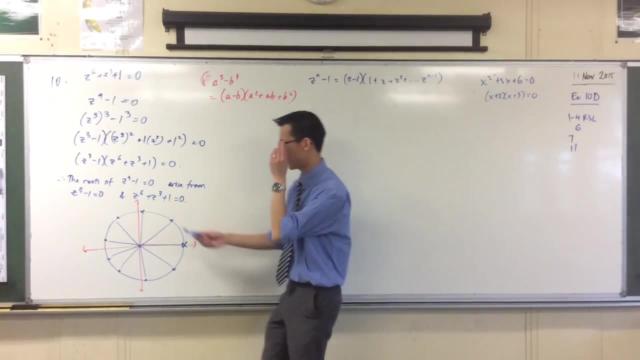 look, at least at least reasonable, okay. So I think we want to do that. Okay, now I've got all the ninth roots of unity on there. I want to indicate which of them are solutions to this one, okay. 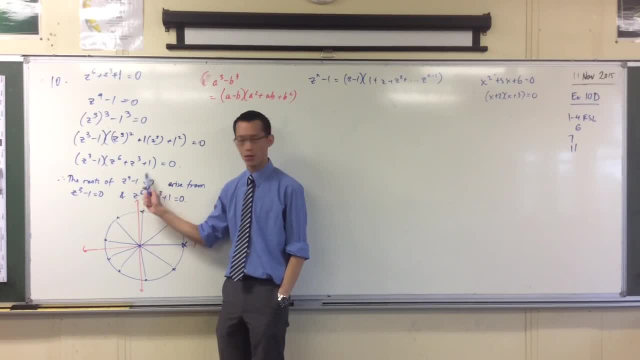 Now, in order to think about that, remember what I just said: All of the ninth roots of unity are either solutions of this or they're solutions of this. okay, Now, this is just the cube roots of unity. I know them. 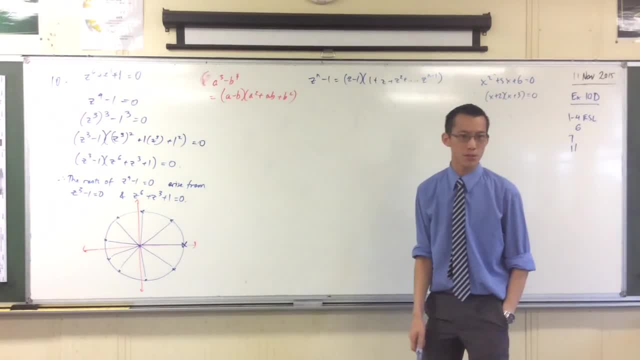 I know them really well. actually, Which of these three are the cube roots of unity? if I label them out, What's the first cube root of unity? That one, The first one, is just one, So I'm going to call that. 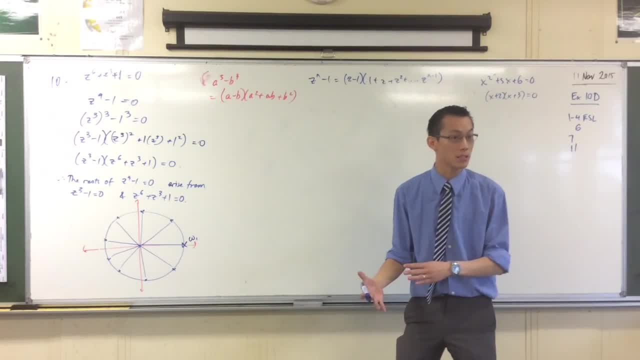 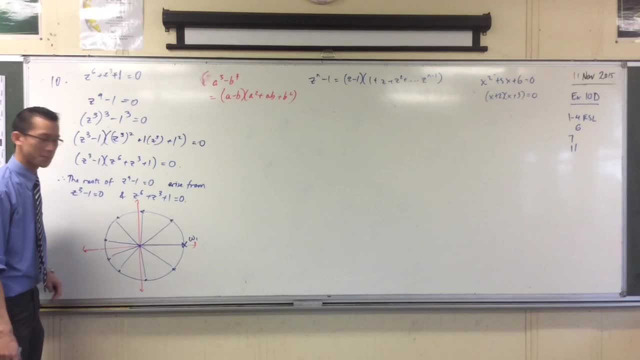 omega one. okay, Because I actually don't want these solutions. I want these solutions, so I'm separating out these solutions, right? Where are my other two cube roots of unity? Yeah, they're going to be these two guys, right. 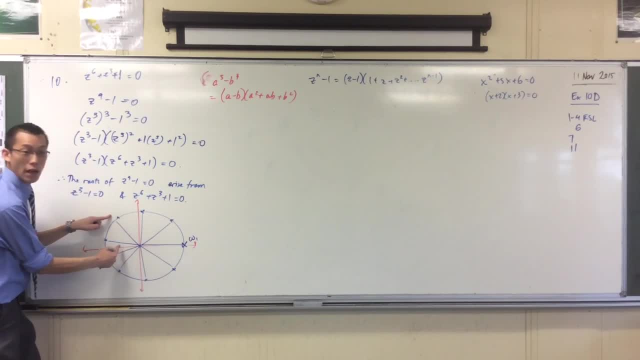 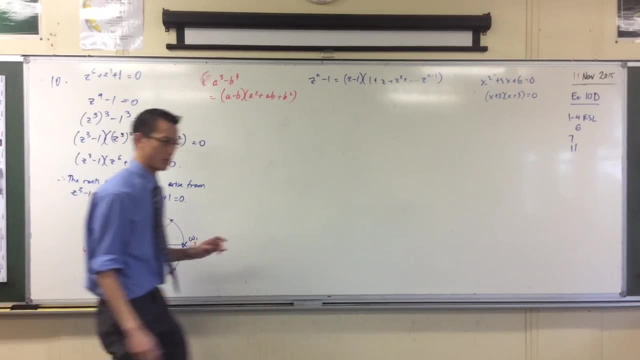 That would be two pi on three to get to here and this would be minus two pi on three. So I'm going to call this one omega two and that makes this one omega three, Not to be confused with the fatty acid. Okay now, 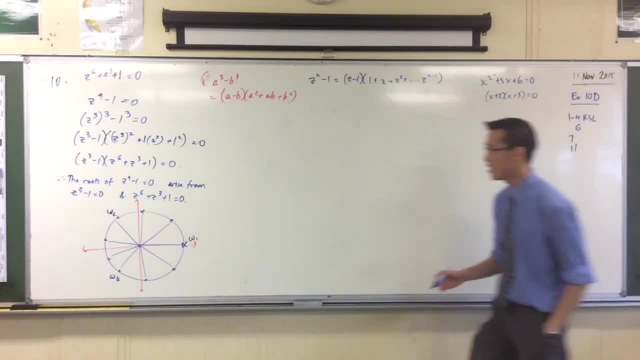 those are the roots I don't want. Those are the cube roots of unity, okay. So I'm just going to say: you know, these solutions or these roots are the omegas, okay, So I separate them out and these guys. 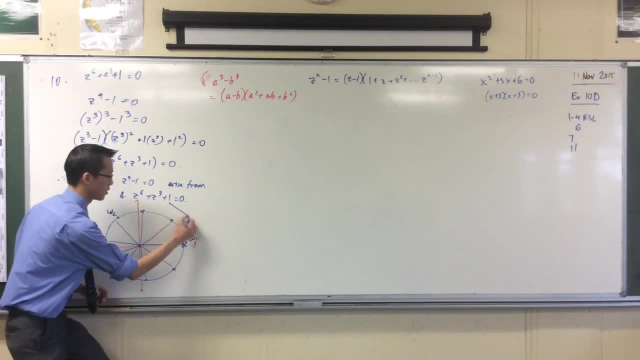 I'm going to call them the zeds, the zed ones and two. They're the ones I'm actually after. okay, So I'm going to say here the solutions are zed n. Okay, So I can simply end with another colour. 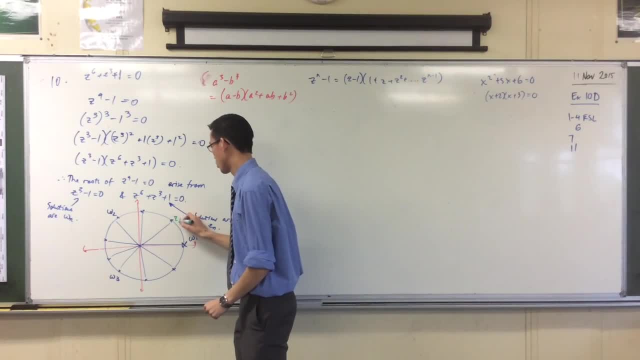 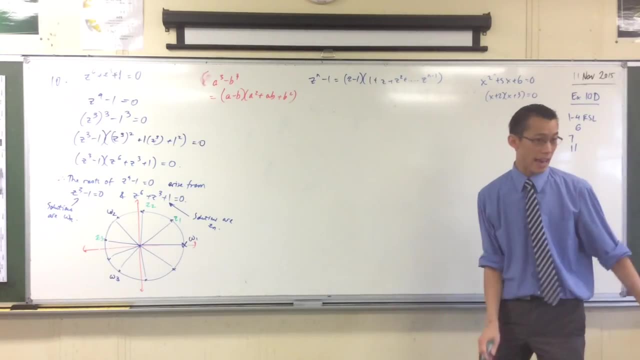 because I've got them. I'm just going to name which ones they are. There's zed one, there's zed two, there's zed three- and you'll notice, because I've taken unity out of the equation- the remaining roots. 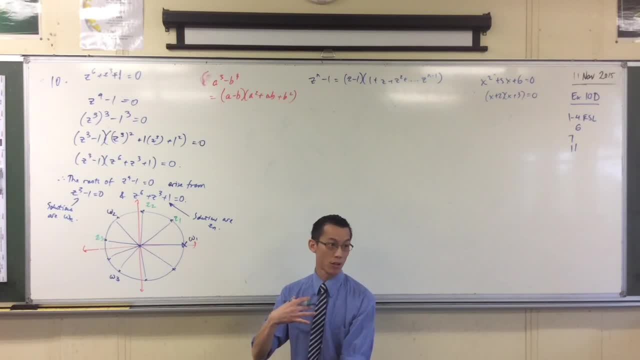 are all complex conjugates. okay, So just to help me later on, this is going to be very, very useful for me. Not only am I going to call this zed four, I'm also going to note that it is the conjugate.